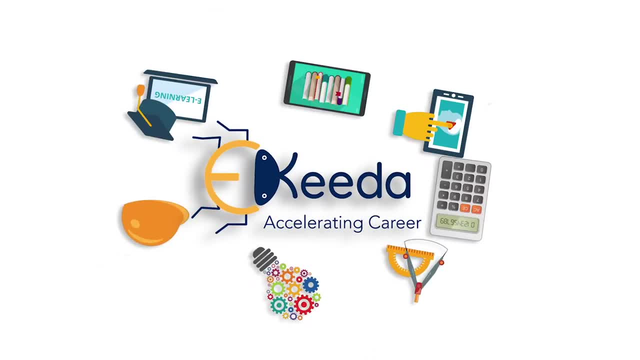 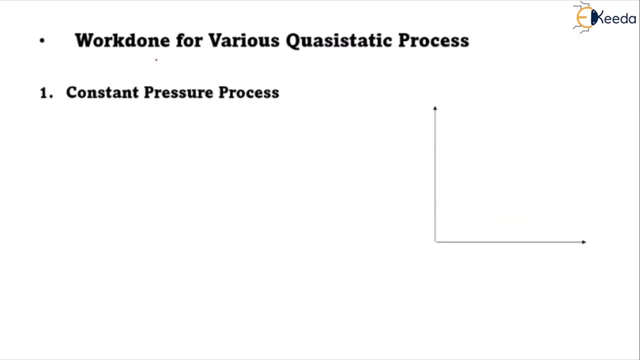 So let's start the discussion of work done for various quasi-static processes. So, as we know about the quasi-static processes which is related to equilibrium condition and in equilibrium condition at each and every state, we will consider the variation in characteristics and properties. that is same, And if we talk about work done, so work done will be the 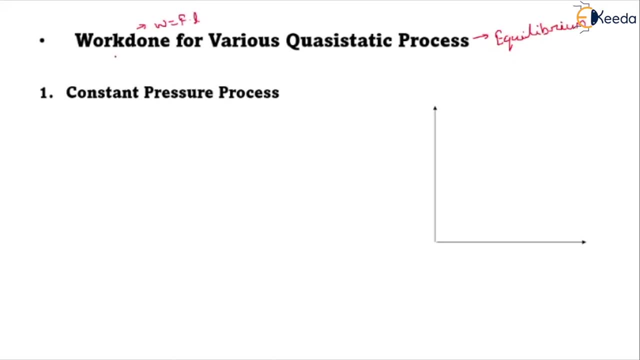 product of force and displacement. So here we have to define the work done for various quasi-static processes. Now, before going to learn about the work done for quasi-static processes here, first we need to learn about different quasi-static processes. So one: 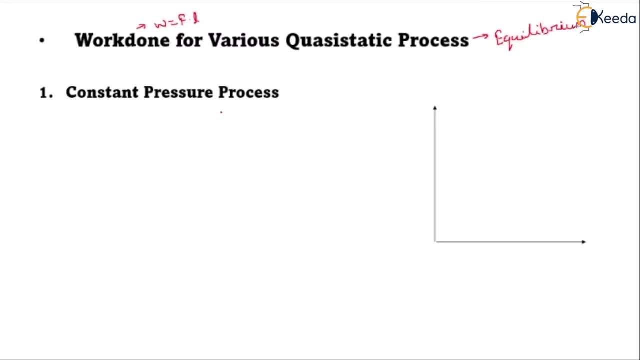 by one, I will teach you about different quasi-static processes. So in this case I am going to correct you of creating two work done. So there we have to define the work done in previous case carefully. let's sew both the work done. So I am going to give you the. 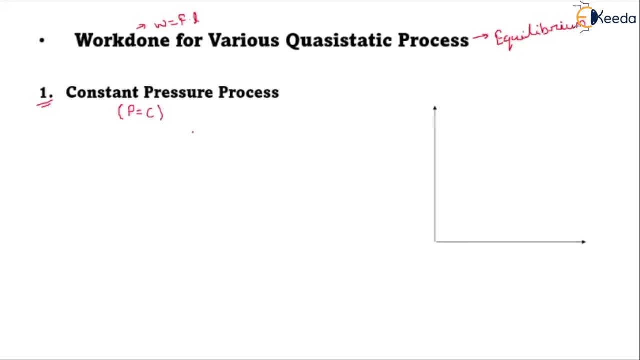 work done so on. So we're going to start with the very first work done so, which is written there for the feature of immobilized partial equilibrium. Now what we are interested, and here this isobaric process we usually define on a particular graph of pressure volume. 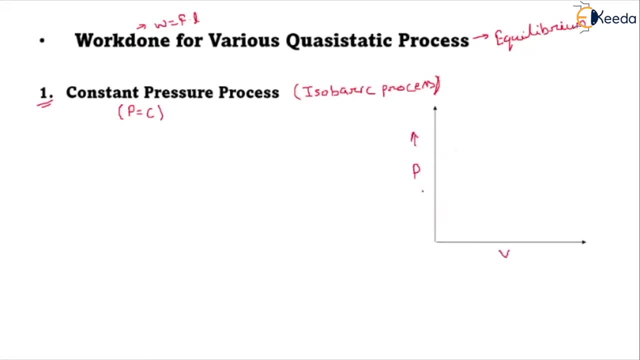 So suppose if we have a graph where the vertical side is represented as pressure and the horizontal side is represented as volume. So here suppose, if we have two states, one is the initial state 1 and another is the final state 2. So here the constant pressure. 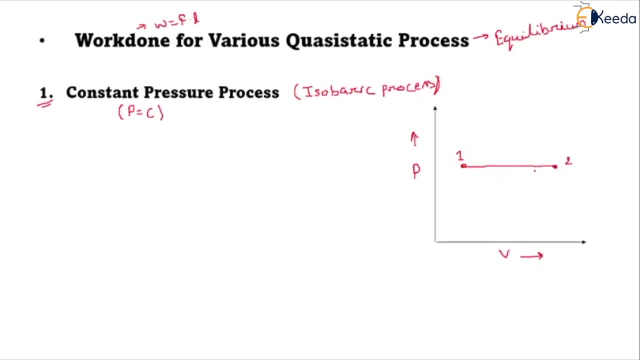 process will be represented by a straight horizontal line. So at this point, suppose, if we have pressure P1 and at this point we have pressure P2. So P1 will be equals to P2 will be representing the constant pressure process. So in this context, 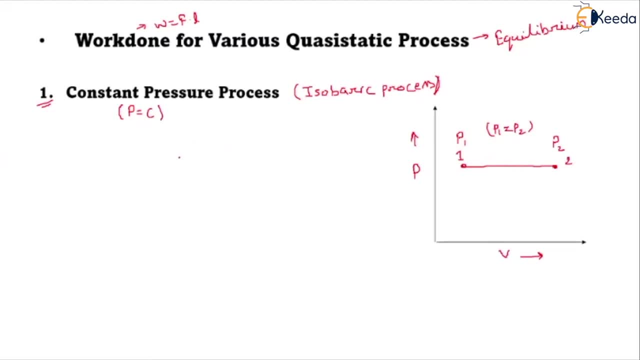 the pressure will be constant. Now, here, this is about the constant pressure process, where the pressure is constant throughout the process. So this 1, 2 is represented as a process and pressure at each and every point will be same. So this condition is represented as: 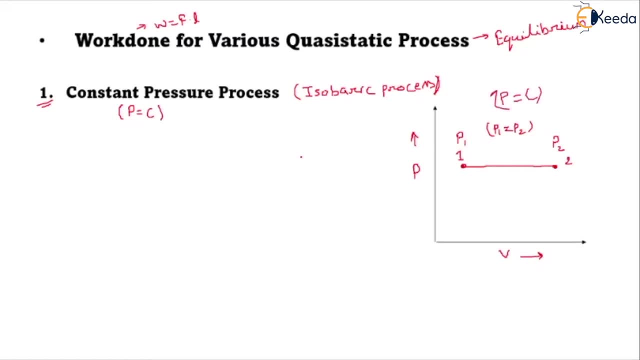 pressure equals to constant process. Now here, if we want to define the work done, So let us define the work done for this. So work done. we usually define. suppose our process is process 1, 2. So it will be W1, 2, and here we are considering. 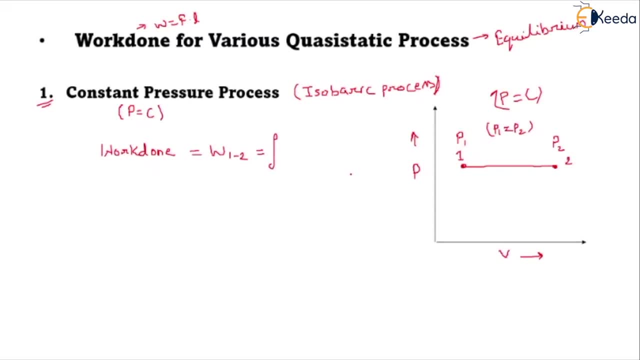 quasi-static process, So it will be under thermodynamic equilibrium, So it will be represented by displacement work. So W1, 2, integration of 1, 2, 2 PDV will be our work done for the constant pressure process. Now here, if we simplify this term, So the pressure, 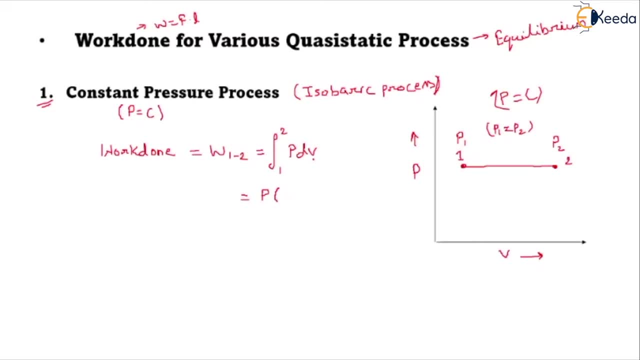 is constant throughout, and here integration is with respect to V, So it will be V2 minus V1. So this will be the formula of work done for constant pressure process. So this is representing the work done for the constant pressure process and this term is representing the 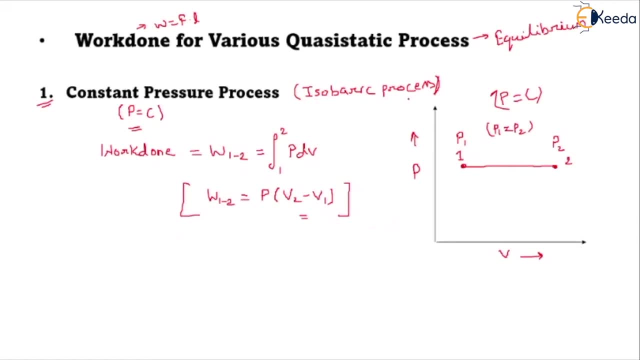 constant pressure process or isobaric process. So this is a first quasi-static process and work done for this. Now if we want to define the work done on this graph, So here we have constant pressure at 1 and 2, both point. So here if we want to define the work done for this constant 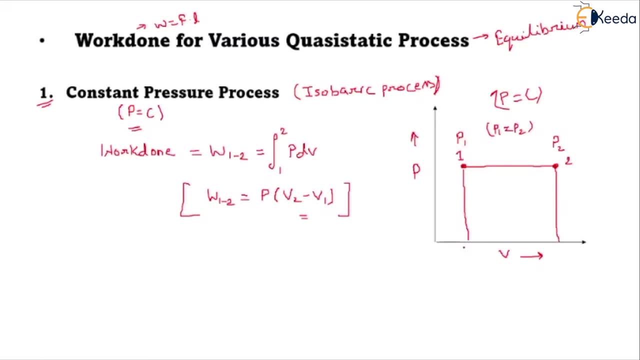 pressure process. So here volume is variable. Suppose volume V1 here and V2 here. So this complete area under the constant pressure process. So here we have constant pressure at 1 and 2.. So this complete area under the graph 1,2 or under the line 1,2 will be represented as work done. 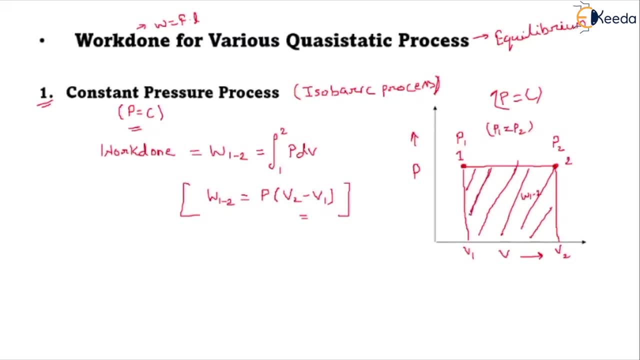 for this constant pressure process. So either we can define work done with the help of graph or we can define work done with the help of this equation. So this area, under this graph, will be represented as work done for constant pressure process. Now let us discuss another process, that is, constant volume process. So here, as per name, 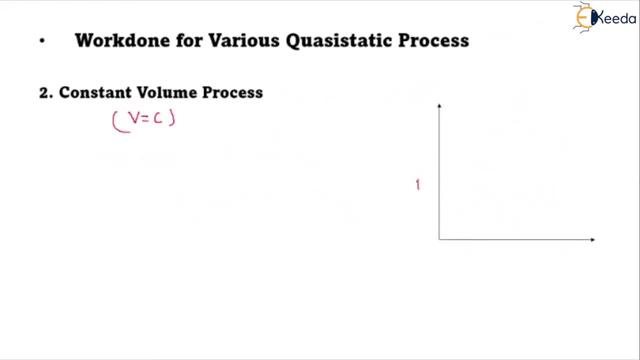 here. So suppose if we have a graph, PV diagram, and we have two conditions, 1 and 2.. So, as per the constant volume concept, this line, or the states which is representing initial and final state, is represented by one vertical line. Suppose this is initial state, this is final state. 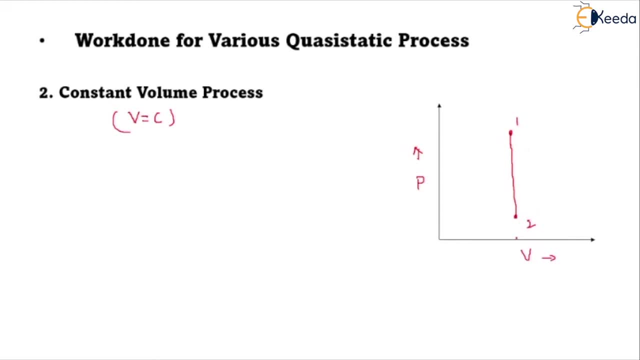 So at this point this volume- suppose at this end we have volume V. So this is representing the volume is constant at this point. here we have volume V1. at this point we have volume V2.. So V1 will be equals to V2, equals to V. this is the condition of constant volume process and 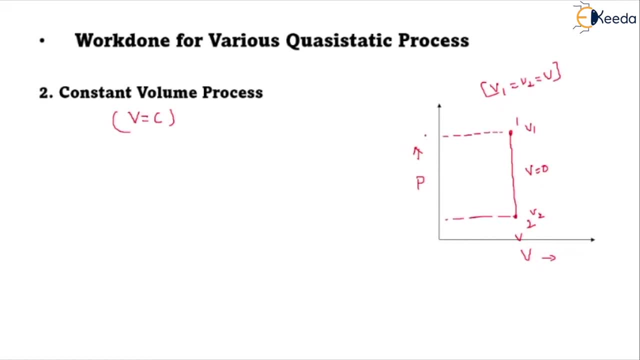 pressure will be vary. Here pressure can vary, but the volume will be constant. So this is constant volume process and it is also called isochoric process. It is called isochoric process Now here if we want to define the work done for. 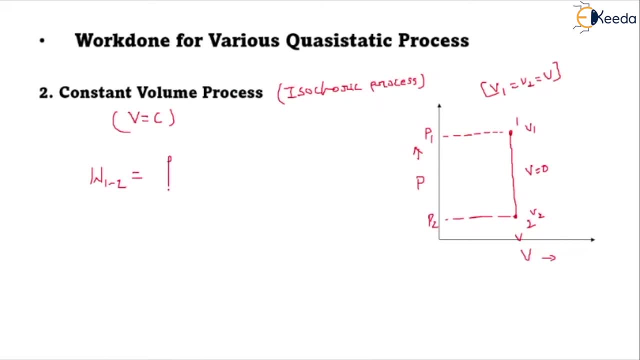 this isochoric process. So work done, simply it will be represented by displacement. work done, PDV Now, if we simplify this. so here this V1 and V2 are representing the volume change which is constant. So here, if we want to define the change in volume, So change in volume will be represented. 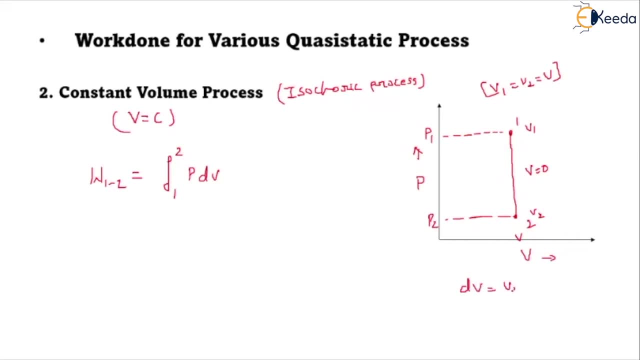 by DV, So it will be equals to V2 minus V1.. So V2 and V1 is same, So it will be 0. It means this term will be 0. So if we simplify this, so it will be PDV. 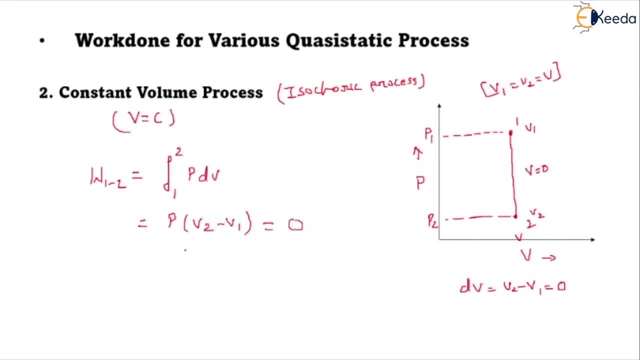 V2 minus V1.. So this complete term will be 0.. It means the work done for this particular process will be 0.. PV2 minus V1 will be 0.. So W12 will be 0 for this process. In that case we cannot define. 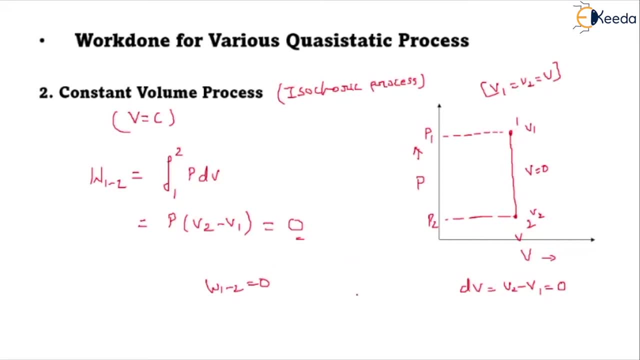 the area for the work done in this case, because W value is 0. So it will be represented by straight line. So this is about the constant volume process. Now let's decide the work done for this particular process. So if we simplify this, so here this: 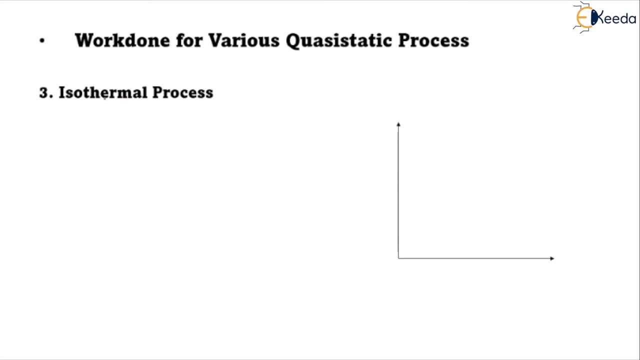 is the first process, So we will discuss the third process, that is, isothermal process. Now, isothermal is what It is called reversible isothermal. So in that case temperature will be constant. So pressure will be varying, volume will be varying, but temperature will be constant. 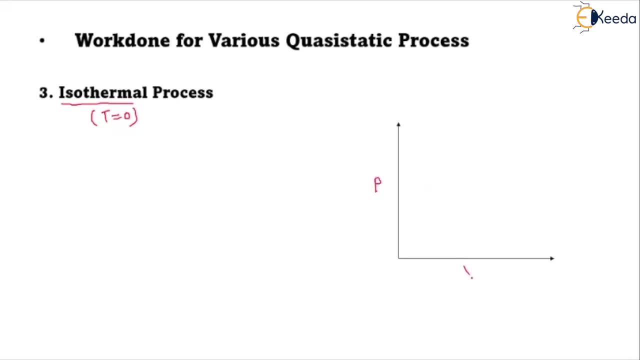 So here, if we are going to define this graph with pressure volume, So it is called pressure volume diagram. So in that case, what will happen? This particular process will be defined as P, V equals to constant. So here, if we define this as 1 by V multiplied by constant. So here this: 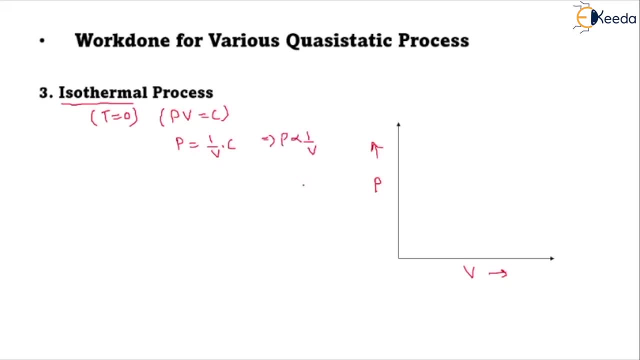 particular term is representing: pressure is inversely proportional to volume, or volume is inversely proportional to pressure. So when the pressure is increasing, volume will decrease, or when the volume is increasing, pressure will decrease. So both are inversely proportional to each other. So here we can say: suppose if we have initial condition 1 and final condition 2.. So if the 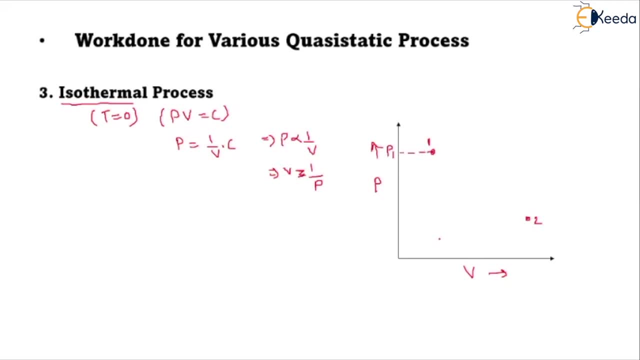 pressure is P1.. So pressure P1 is at higher side and pressure P2, this particular pressure P2- is at lower side. So volume at point 1 or state 1 will be lesser or at lower side and volume at point 2 will be at higher side, V2.. 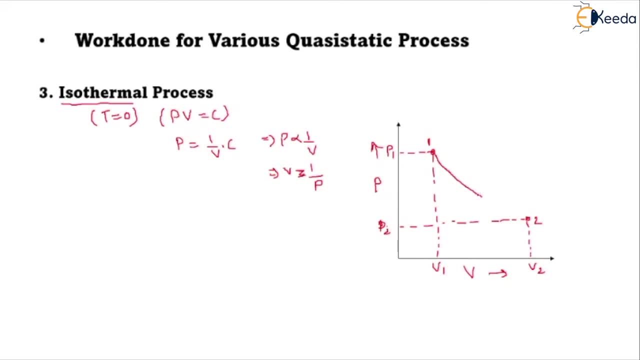 So in this case a graph should be like this: It will be represented by a curve, So this graph is represented as P, V equals to C. So in this case, if we want to define the isothermal process, So isothermal process will be represented by P, V equals to C, And this process is also called. 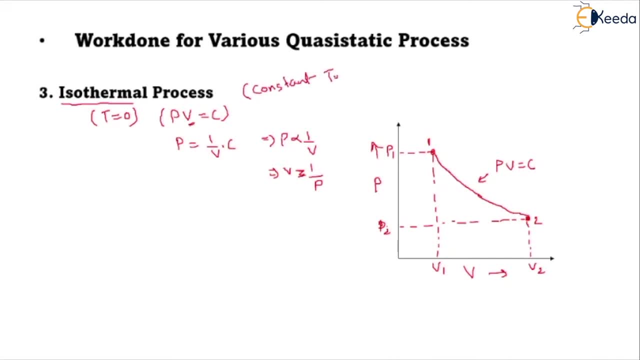 constant temperature process. So it says that the temperature is constant. So this is about the isothermal process. Now we want to define the work done for this isothermal process. So work done. W12 for this process will be what It will be represented by PDV from 1 to 2.. This is the same displacement work. Now here. 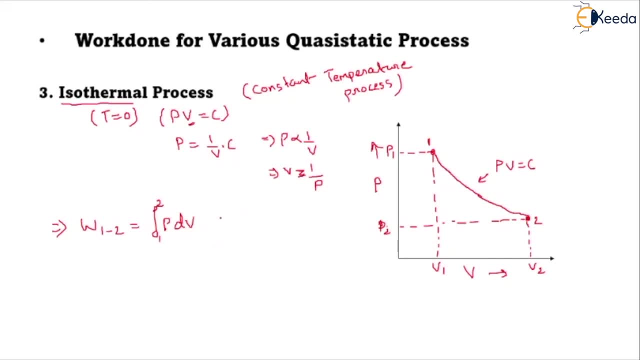 what we will do Here. initially, we need to define the value of p. So how we will define the value of p. So the value of p we will define here. as we know, pv equals to constant. So in that case we can write down this term as: pv equals to p1, v1 equals to constant and that is further equals to p2- v2.. 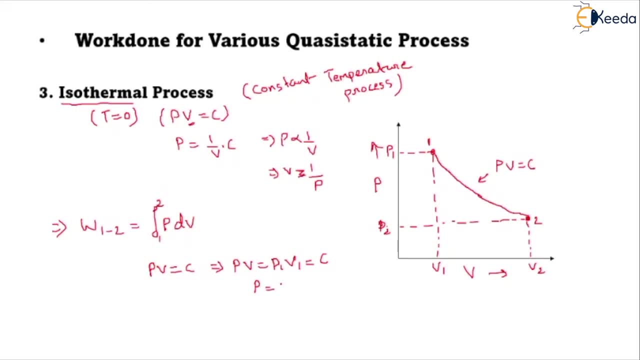 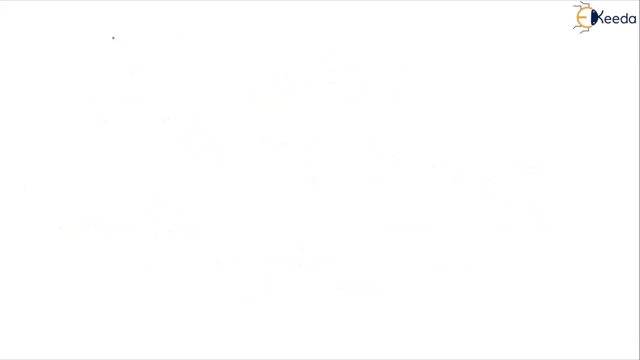 So this p we can write down as p1, v1 by v. So suppose this is our equation 1.. So we can have this value of p with the help of this equation. So we will put this value here in this equation. Now, after putting this value, what we will get, So the w12 for the isothermal process, is: 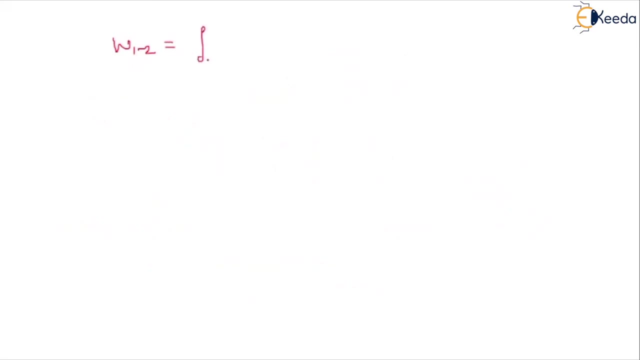 it will be integration of 1 to 2, p1, v1 by v, dv. So this will be our equation. Now we will simplify this. So p1 and v1 will be constant. So here what we will do: We will integrate 1 by v with respect to v. 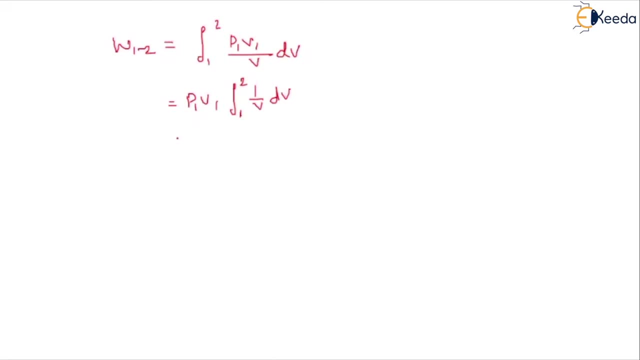 for two condition: 1 to 2.. So it will be what After integration? we will get p1, v1, log of p1, v1 by v. So this will be our equation. Now we will simplify this, So p1 and v1 will be. 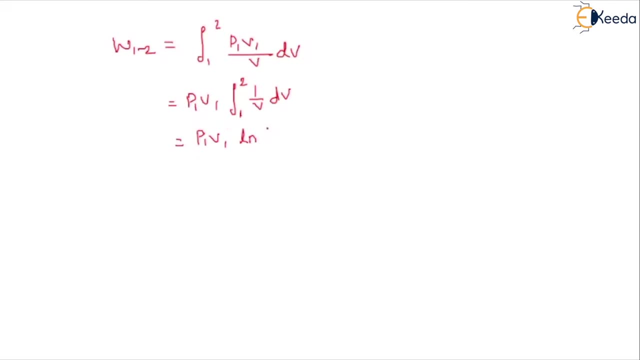 log v2 by v1. It will be log v2 by v1 or, in case of p, we can write down this as p1 v1 log p1 by p2.. So these two equations are representing the work done for this isothermal process and how. 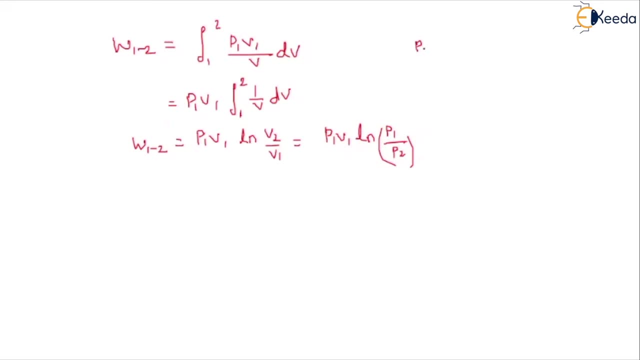 we are getting this p1? So p1- v1, that will be equals to p2- v2.. So p1 by p2 will be equals to v2 by v1. So with the help of this term we can define this equation. So p1 v1 log v2 by v1, or p1- v1 log p1 by p2, will be our work. 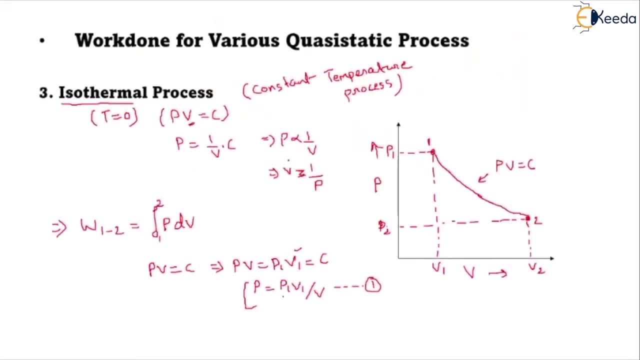 done for isothermal process. Now, if we want to define the work done for isothermal process, then we have to define the work done for isothermal process. So, as for the concept, the area under this graph will be represented as p1, v1, log, v2.. So this complete area. 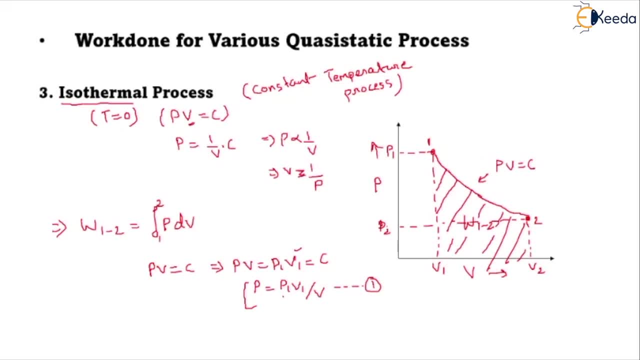 will be represented as work done for the constant temperature process or reversible isothermal process. Every process will be reversible in quasi-static process. So this is about the third process, that is, isothermal process. Now let us discuss the fourth process, which is very important process. it is called polytropic. 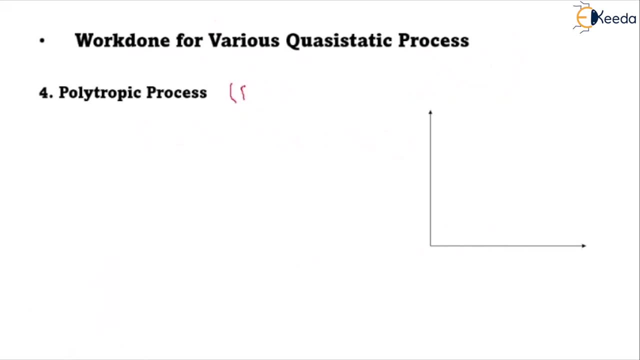 process, So polytropic process, where the pressure and volume vary, and it will be equals to pv, to the power. n equals to constant. So this term is defining the polytropic process. Now this n? n value is constant everywhere. So on the basis of n value we can define the graph of polytropic. 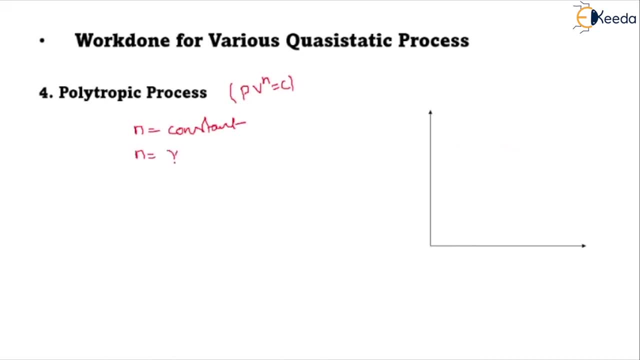 process. Suppose n value is equals to gamma, where gamma we define on the basis of specific heat or the ratio of specific heat at constant cp by cv. So cp is representing the pressure- constant pressure- and cv is representing the constant volume, So specific volume at constant pressure. 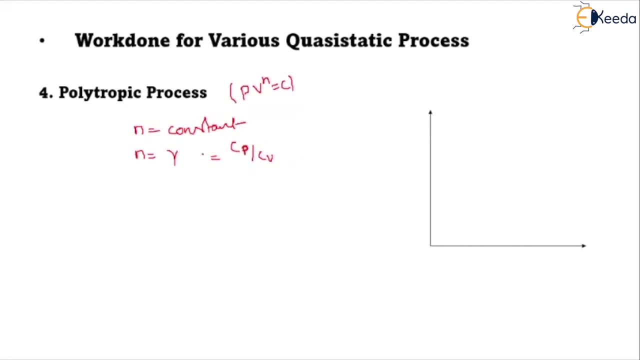 and constant volume is equal to pv. So this is the graph of polytropic process. Now let us volume. ratio is representing the value of gamma. So this particular process will become adiabatic process. It is represented as adiabatic process. How adiabatic process is defined. 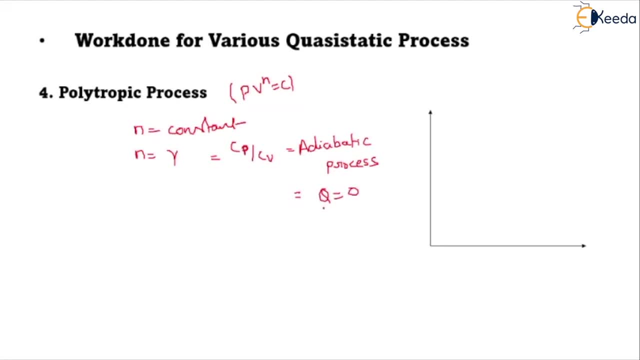 Adiabatic process where the heat transfer is zero, Q value is zero, So that particular process is adiabatic process. Suppose if we have any system and the system is insulated, So neither the heat is transferring to from system to surrounding. 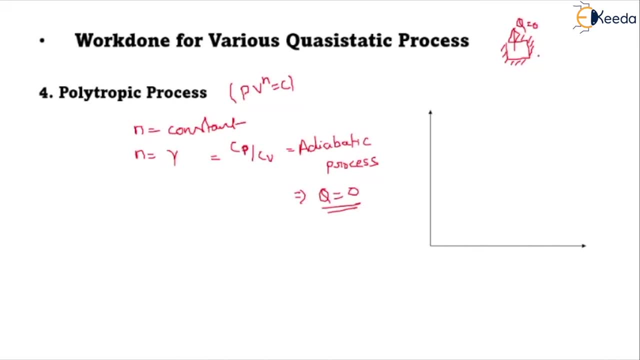 So it will be zero. or surrounding to system, So that will also zero. So it is representing the adiabatic process. Now let us discuss again the polytropic process, which is represented as pv to the power. n equals to c, So n value will vary and the graph is coming accordingly. 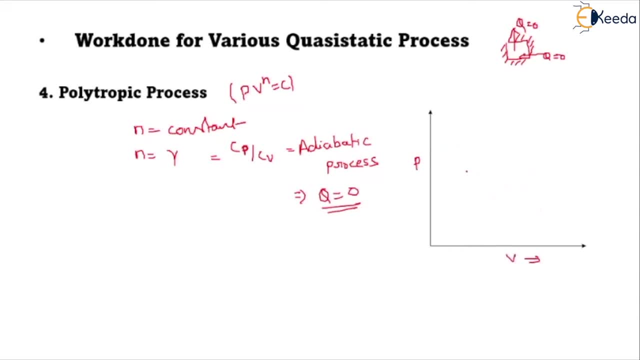 So here we have pressure volume graph and we have two states, one and two. So this is our initial state, This is our final state. So in this condition we will have value p1 and at second state we will have value p2.. At final volume, we can define as v1 and at this particular point we 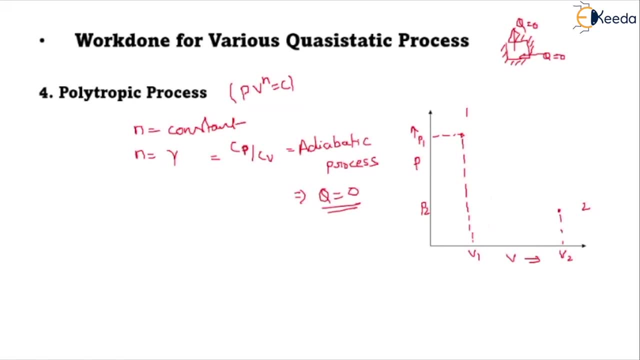 will define value v2.. So here this graph is represented as pv to the power, n equals to c. So here this graph should be like this: It will be as per the curve, and this curve we will get as per the value of pv and n. So this will be pv to the power, n equals to c. Now here let us discuss this term. 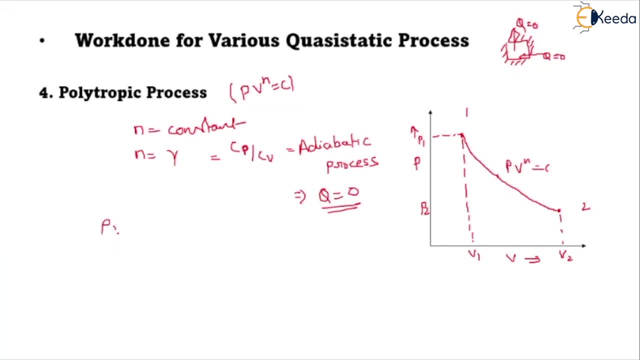 pv to the power n equals to c. So pv to the power n equals to c. So it will be equivalent to p1, v1 to the power n, or it will be equivalent to p2, v to the power n or other terms if involved. so it will be continued. So here we have this term Now on the basis of: 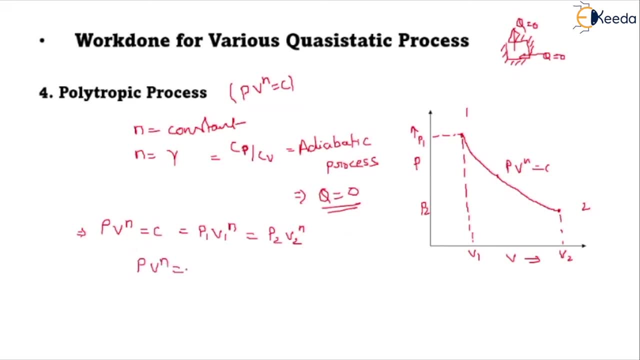 this equation. we can write down this: p v to the power n equals to p1 v1 to the power n. So it will be equal to what? So p will be p1 v1 by v, that is, to the power n. So here we have the value of p. Now if we want to define the work done for this process, 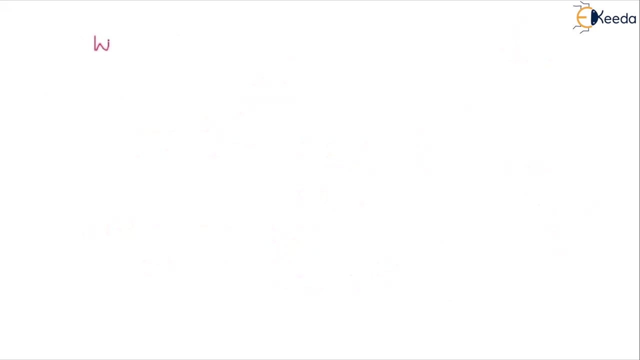 So work done will be same. It will be represented by the displacement work, So work done. So it will be w12 and it will be integration of 1 to 2 p dv. Now we will put the p value here, So it will be. 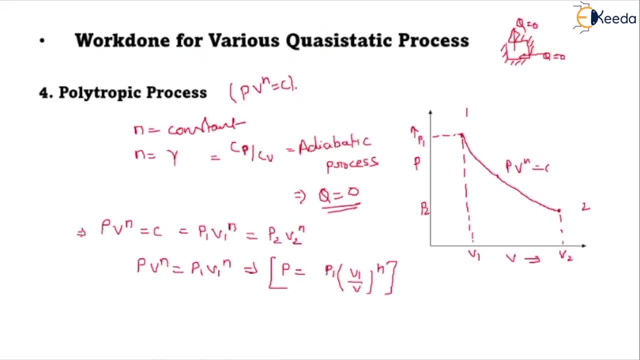 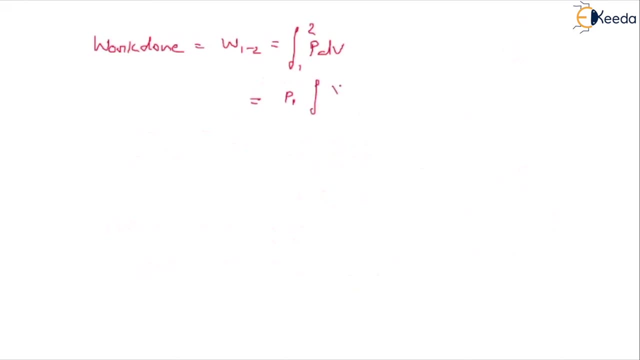 what p1.. p1: v1 by v to the power n, So it will be p1: integration of v1 to the power n divided by v to the power n dv, and the limit is 1 to 2.. Now here we are, integrating with respect to v, So this v1. 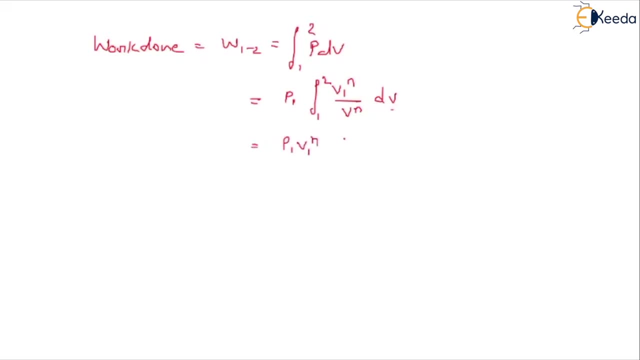 will be constant here, So it will be p1, v1 to the power n, integration of 1 to 2, v to the power n, 1 by v to the power n dv. Now, this term we have to integrate, So it will become minus n when it go on. 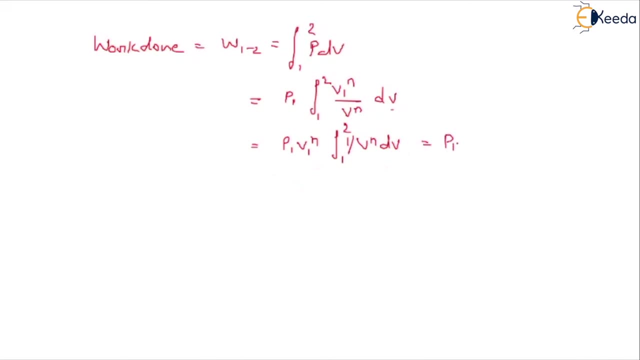 numerator. So this term will be what It will be: p1 v1 to the power n. 1 to 2 v to the power minus n dv. So if we simplify this or if we integrate this, so it will be what: p1 v1 to the power n divided by: 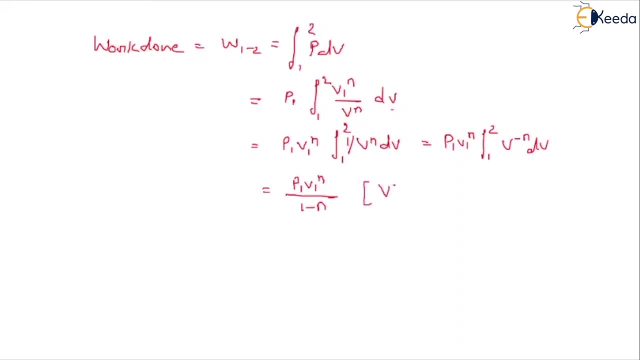 1 minus n, and this term will become v to the power, minus n plus 1 from v1 to v2.. So if we simplify this term, so this term will be what After simplification we will get. the term will be p1- v1 to the power n. 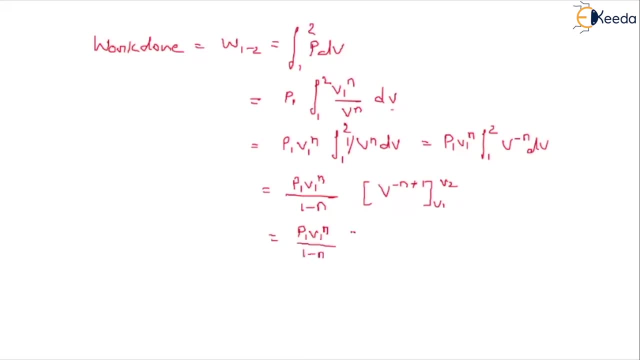 divided by 1 minus n, and this term will become: we will get this term p to the power 1 minus n minus v1 to the power 1 minus n. Now, if we again simplify this, so here we will get p1, v1, p1, v1 minus p2, v2 divided by n minus 1.. After simplification: 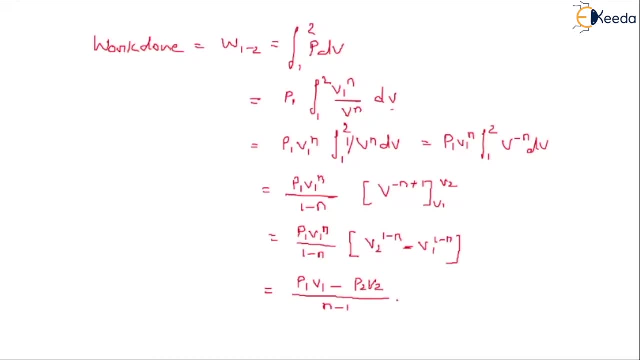 if we open the bracket, so we will get this term. or also we can write down this as: p1, v1 by n minus 1, 1 minus p2 by p1 to the power n minus 1 by n. So here this particular equation: 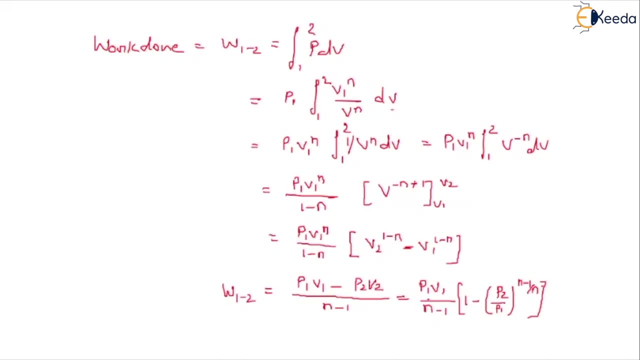 is representing the work done for the polytropic process where n is involved. Now, here, as I told you, if we are considering n equals to gamma, if n equals to gamma and that is equals to cp by cv, so our work done, w1 will be equals to p1, v1 by gamma minus 1 and it will be 1. 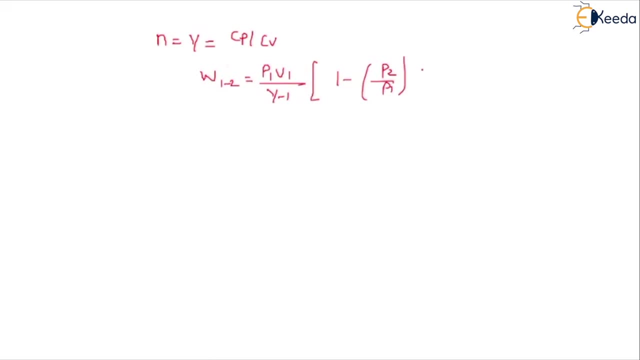 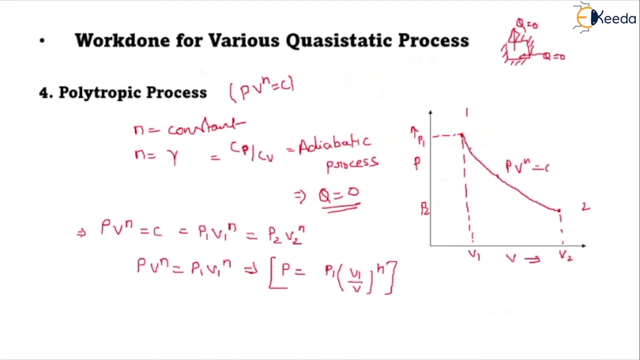 minus p2 by p1 to the power gamma minus 1 by gamma. So this will be representing: is work done for the adiabatic process. Now here. this is the work done in equation form. Now here if we want to define the work. 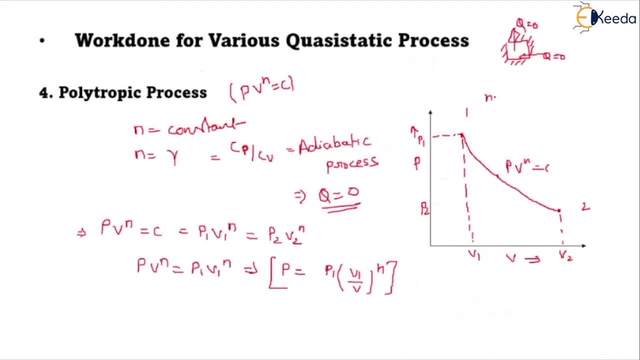 done in graphical form. So here we have to define different values of n. So suppose, if we are considering n equals to 0, in that case n equals to 0. if we put here p to the power, n equals to c, so it will become p equals to c. In that case our graph will be a straight line. So this will be a. 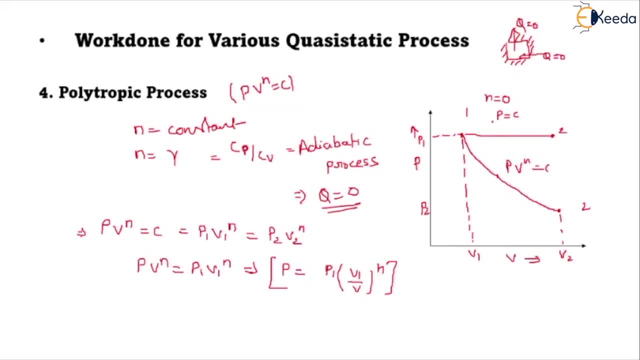 graph. So area under this will be the work done. Now suppose if we are considering n equals to infinite, So our graph will be like vertical line. Now suppose if we are considering n equals to 1, so it will be pv equals to c, where n equals to 1.. So here our graph will be like this. 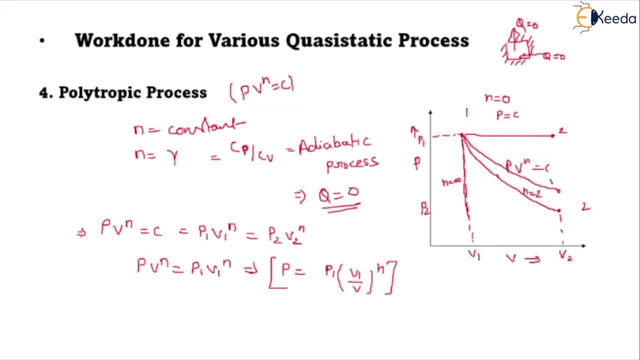 And suppose, if n equals to 2, suppose this is pv. this should be. pv equals to c, where n equals to 1.. n equals to 2, so the variation in property will be different. Suppose if we are considering n equals to 3,, so the variation of 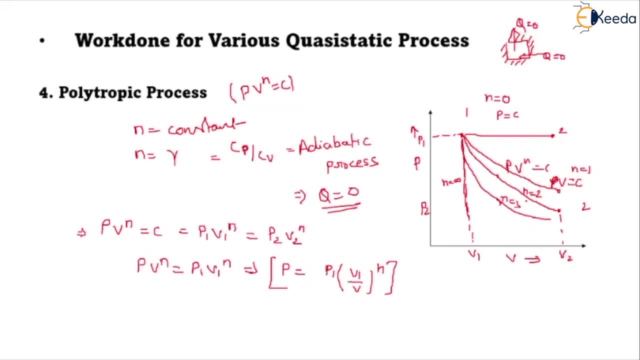 properties will be different. So on the basis of different values of n, we can define different curves for the different polytropic process, or it is also called reversible adiabatic process. So this is about the work done, and if we have number of graphs, so work done inside this particular graph will be. 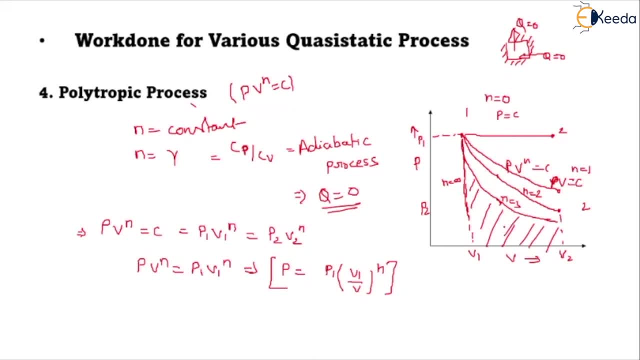 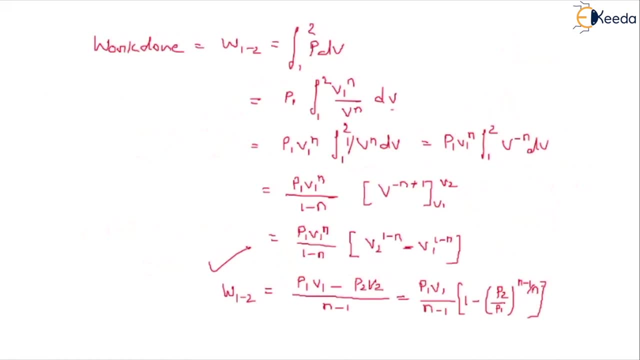 represented as, or this area under this graph will be represented as work done. So this is the polytropic process and this is the formula for the polytropic process. So this is all about different work done for different quasi-static processes. Thank you so much. Subtitles by the Amaraorg community.